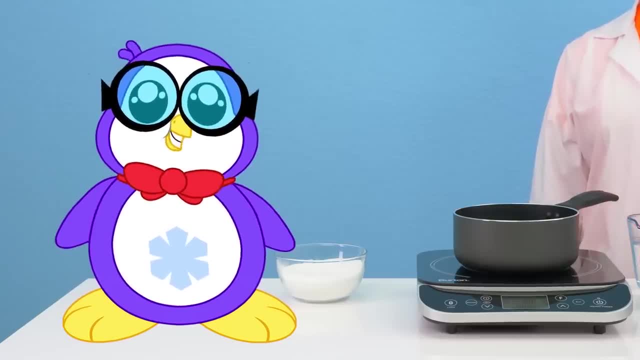 And it looks like geodes, which is cool and it's the best. And it's also on a stick, so it's easy. The first thing that we're going to do is build the very center for our rock candy. Now we are going to use these paper sticks. 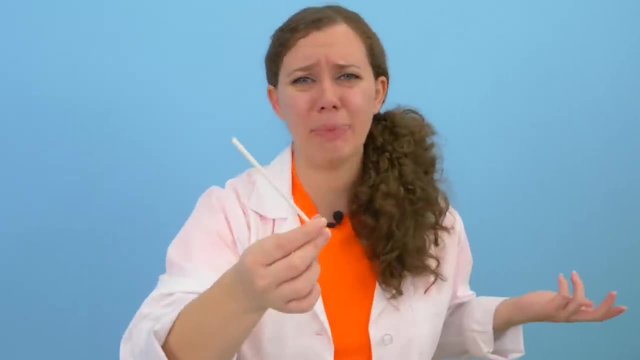 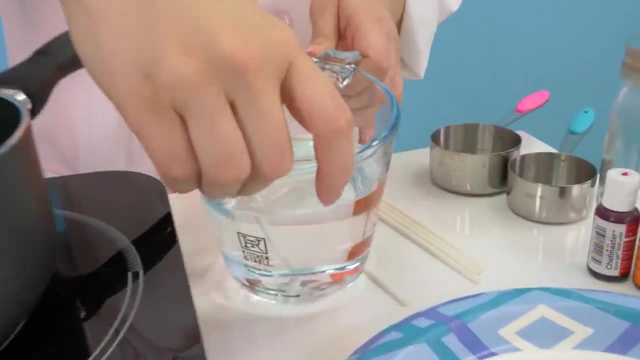 Mmm, paper sticks. You don't eat the paper stick. It's kind of like what would be in the center of a lollipop. We're going to take the stick. we're going to dip it in water like this. Uh well, we need sugar too. We definitely need some sugar, so let's get some sugar on a plate. 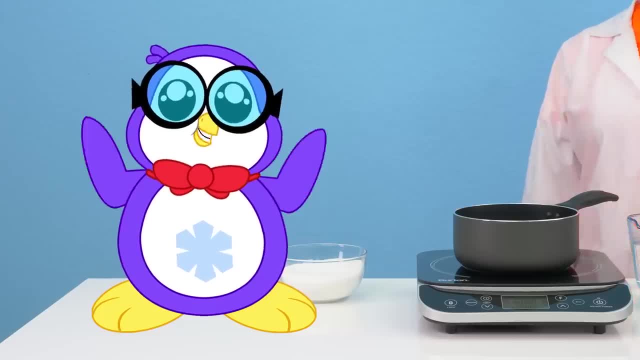 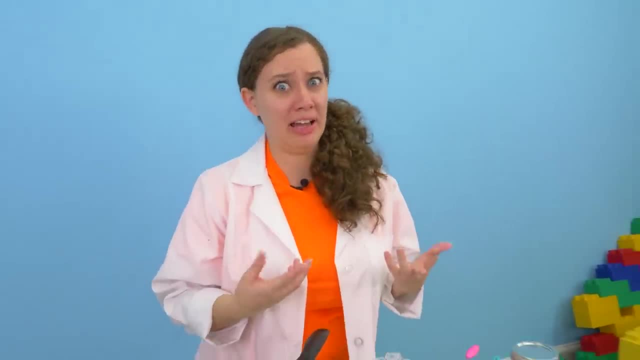 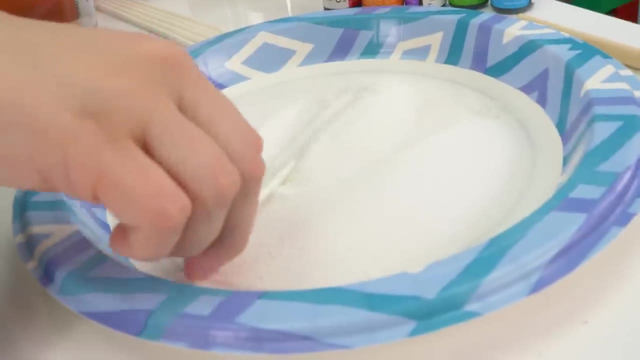 Perfect, Yay, Sugar, Woohoo, Sugar, sugar, sugar, sugar, sugar, Yeah, sugar. There's going to be a lot of that. Now that we have our stick all nice and wet, we're going to roll it around, get some sugar on here. 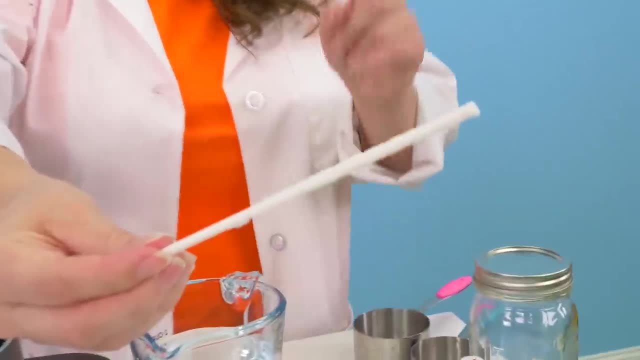 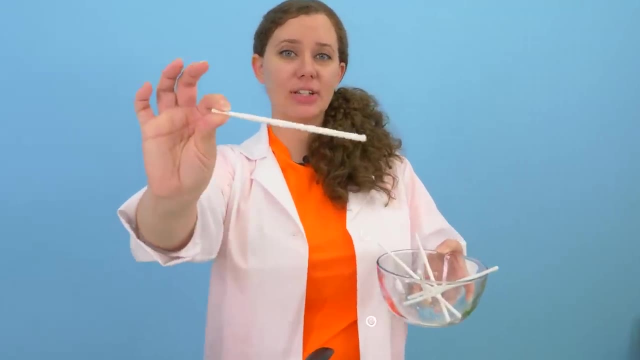 And it should look something about like that, which this will give our rock crystals plenty of stuff to grow on. Now that we have all of our sticks coated in sugar, we're just going to set them aside and let them dry so we can use them later. 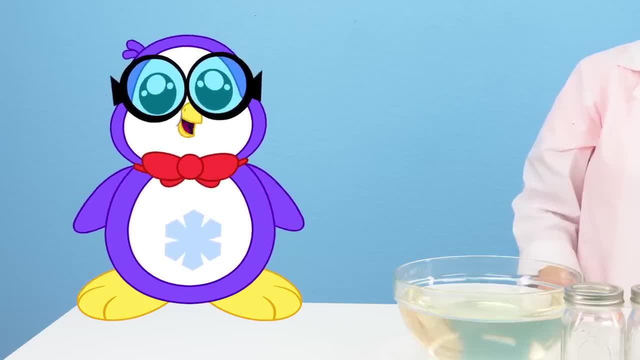 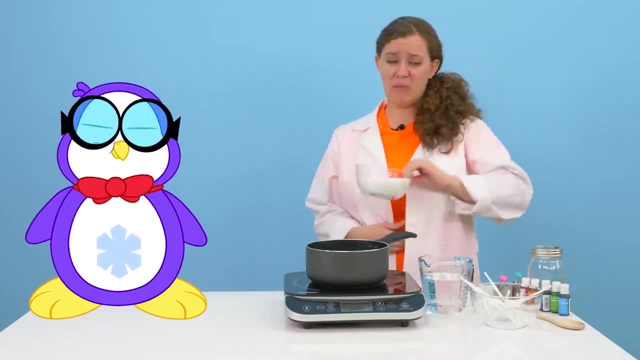 Now we can commence with the creation of our rock candy. Uh, that's right, Peck. Uh, maybe I should just take this sugar away and put it over here. So the first thing we're going to do is add water. 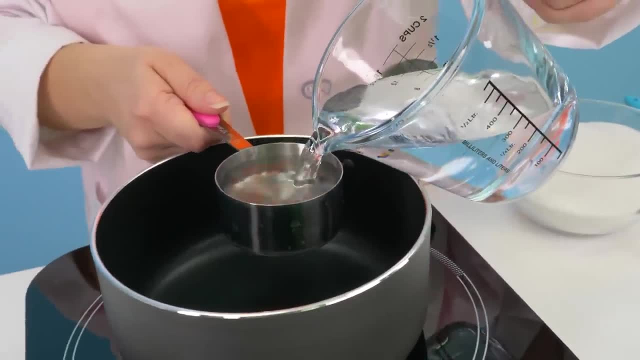 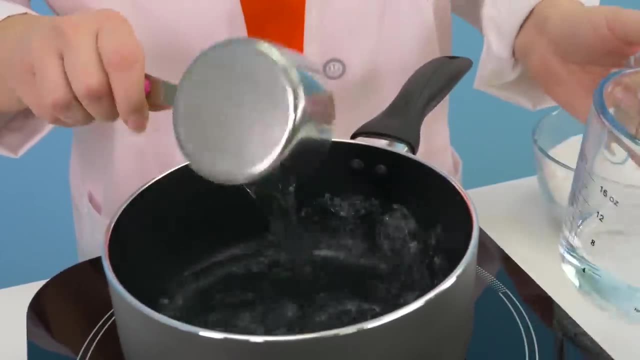 We are going to add one cup of water, which all I could find was a half cup measuring cup, So we need two of them. Then we're going to turn on our cooktop and we're going to turn it on boil so we can get it cooking. 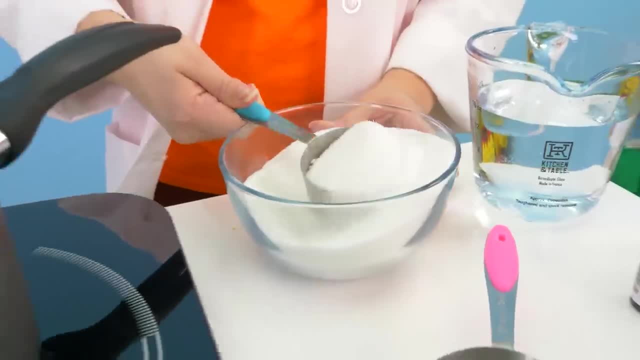 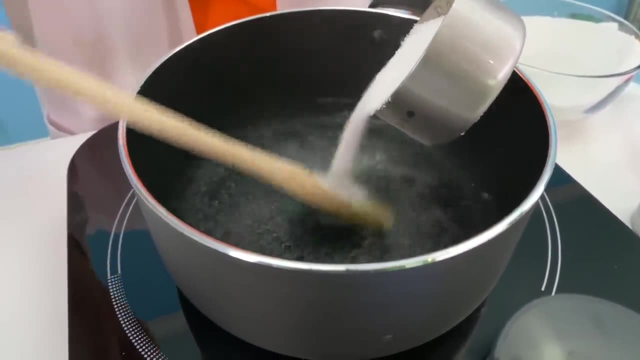 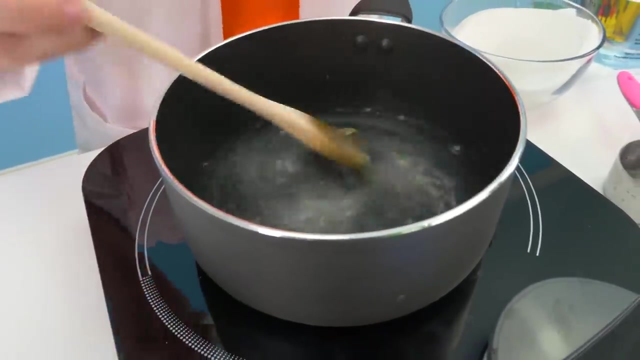 Ah, bubbles. Now we're going to add our sugar. We're going to slowly mix it in. We're going to try to use about two-thirds cup, but we have to make sure it dissolves fully in the water. We have a bowl of sugar water now. 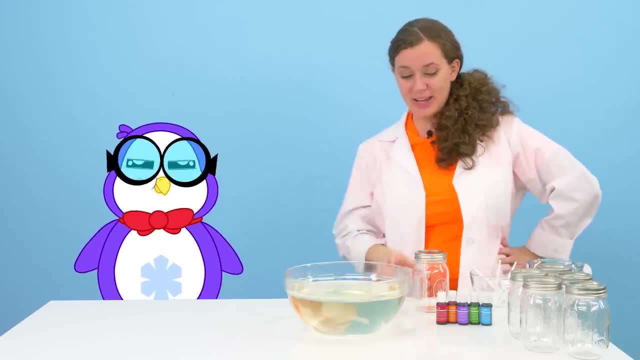 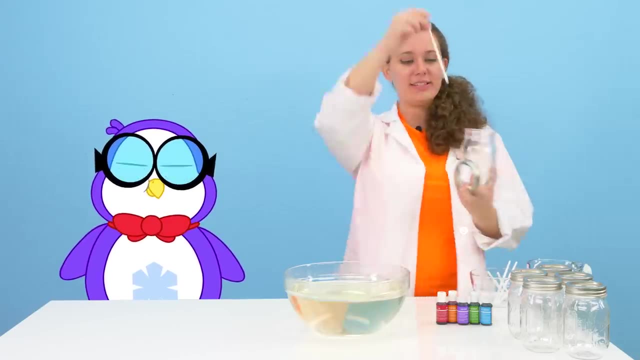 What are those jars for? Well, that is a good question, Peck. We are going to use all these different jars to grow our individual rock candies. Now, we don't need the lid, because this is actually going to go in here just like that and grow all of our crystals. 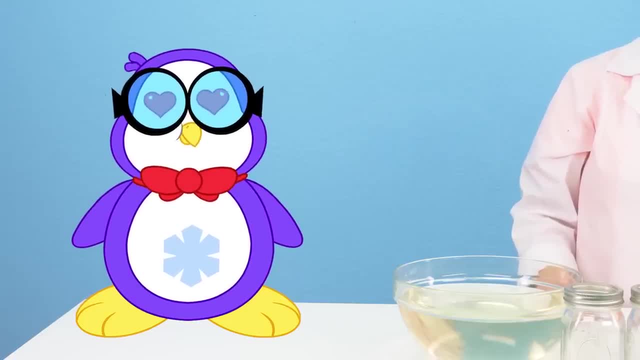 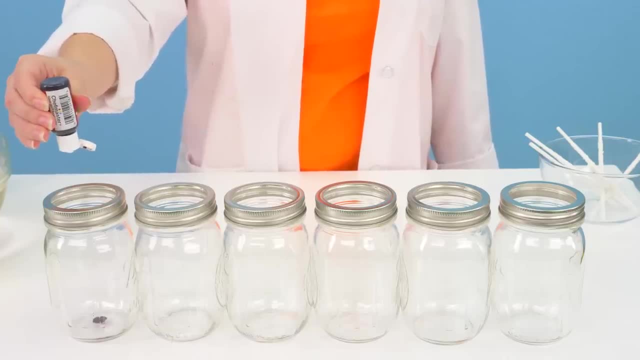 What about the color? I want to see a rainbow. Well, Peck, why do you think I have all this food coloring right here For our rock candy? we're going to make red, orange, green, blue and purple. 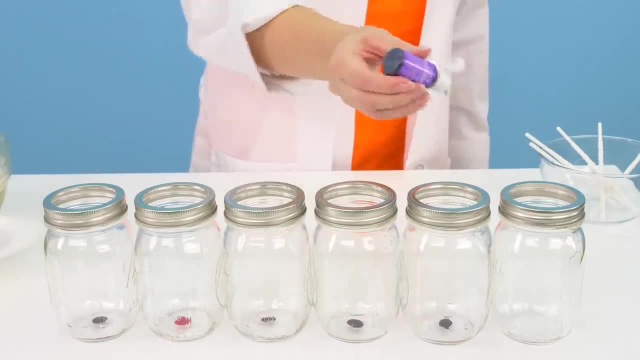 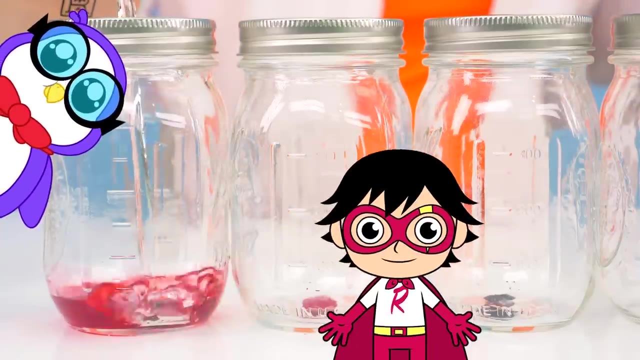 Green, blue, purple, and I think I'm going to leave the last one clear, because I just want to see what the regular rock candy looks like. Red, like Red Titan, cause he's super red. Orange, like Moe- he's so crazy. 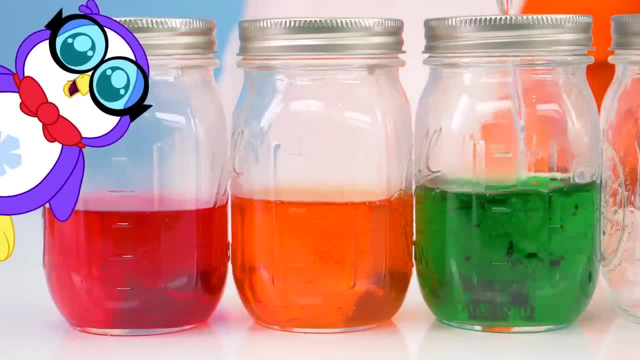 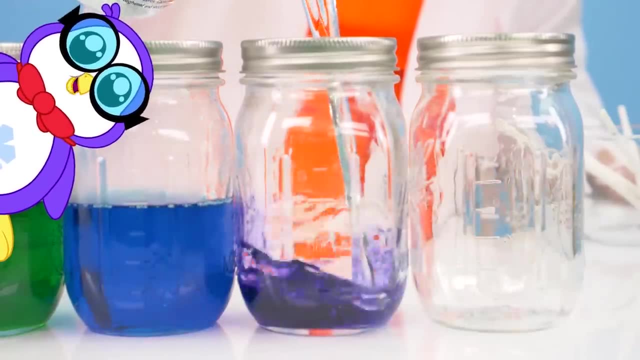 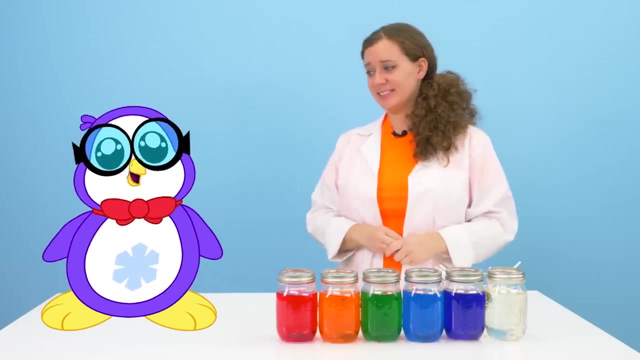 Green like Gus, cause he's a gator. Blue like Gil, cause he's super chill. Purple for Peck, cause purple's the best. See through like a ghost. No, I'm kind of scared. La, la, la la. 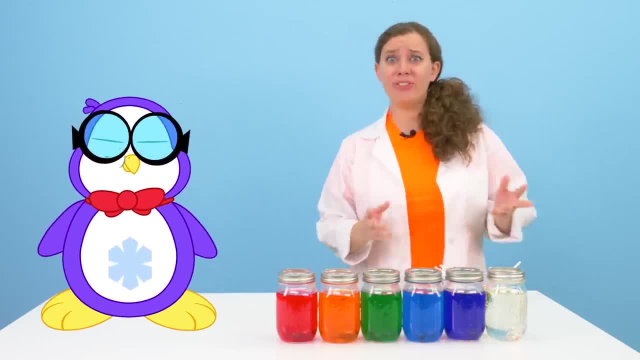 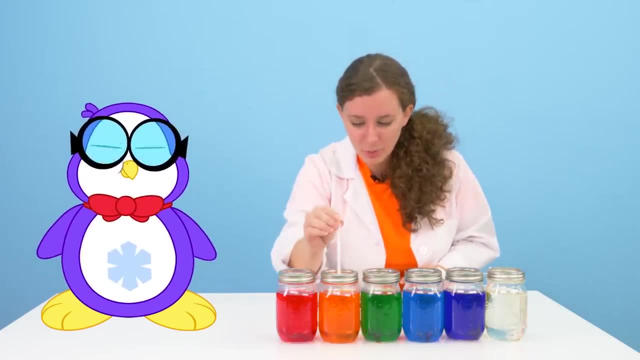 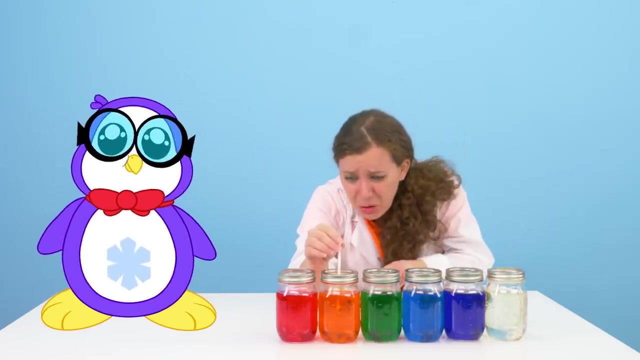 Wow, Peck, that was really something Moving on. the last thing that we have to do to make our rock candy is we just take the center piece, our sugar sticks, and then we just put them right in the center And wait, we need to hold it in place and well, I don't have six arms and if I let it go it's going to fall, and oh no. 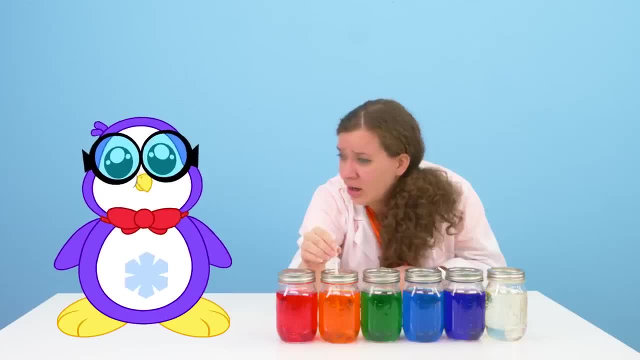 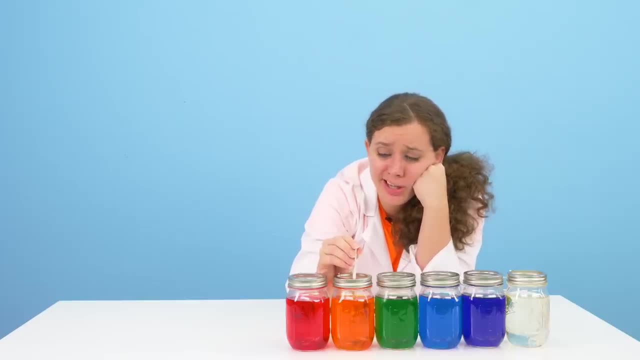 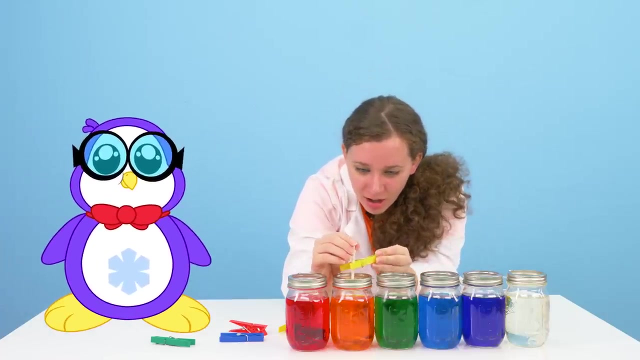 Oh, don't worry, Bree, I know what we can use. Okay, Peck, hurry, Be right back. I sure hope Peck gets here soon. I'm getting so tired. Hey, these are perfect. Oh, that is much better. 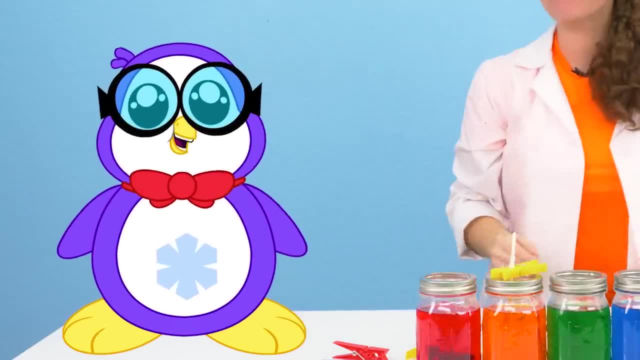 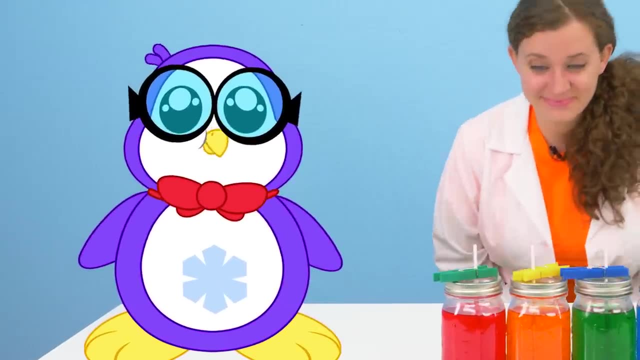 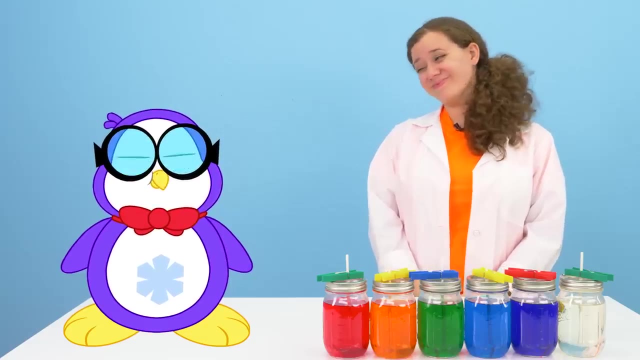 It was a success. Now we can start making the candy. Hmm, hmm, hmm, Oh, ha, ha, ha. yeah, How long do we have to wait, Like five minutes? Oh, I mean 10 minutes, 30 minutes. 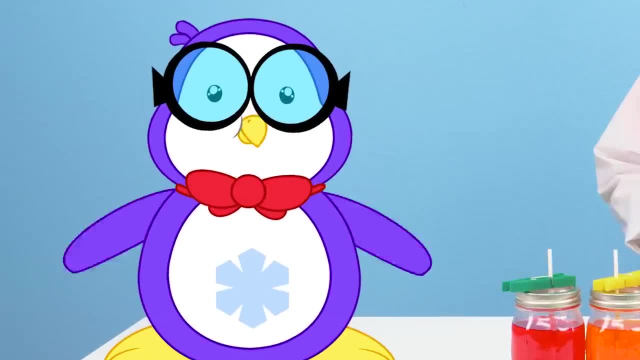 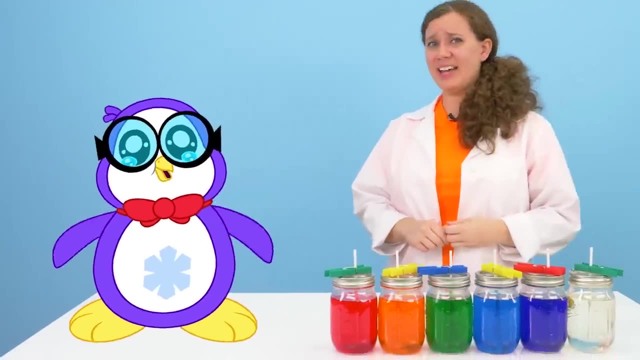 No, Peck, it's going to be more like five days. Five days What? But that's like 7,200 minutes. No, Okay, I'm just going to go. Don't worry, Peck, You got this. 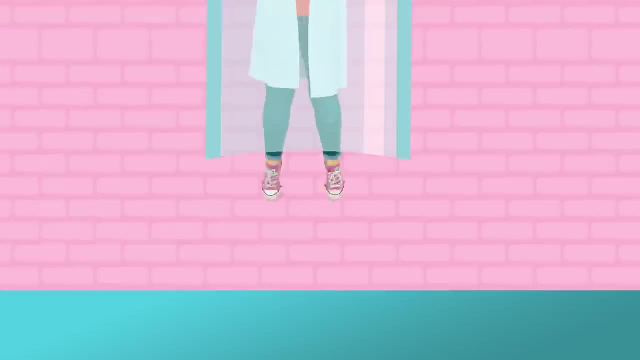 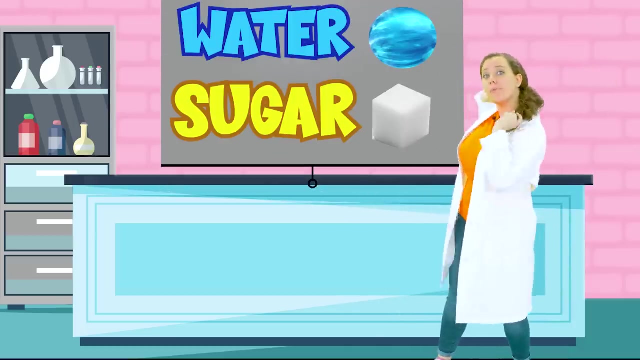 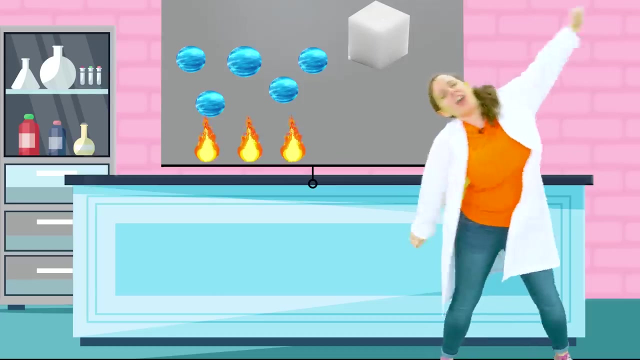 I'll see you in five days. Bye, Wow. Well, since we're just waiting here, how about we take a look at the science behind rock candy? So water and sugar are both molecules. Now, when we heat up the water, the water molecules spread apart. 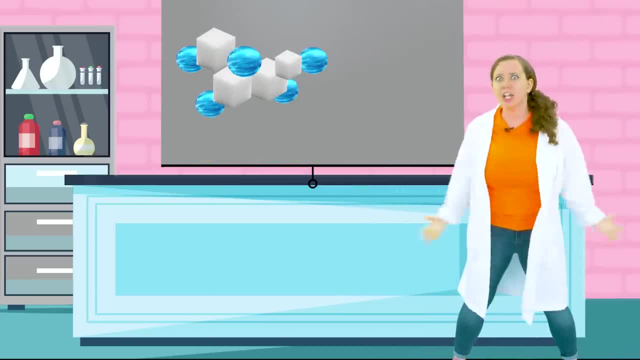 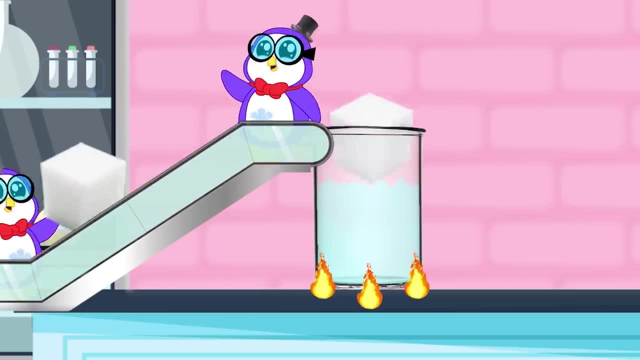 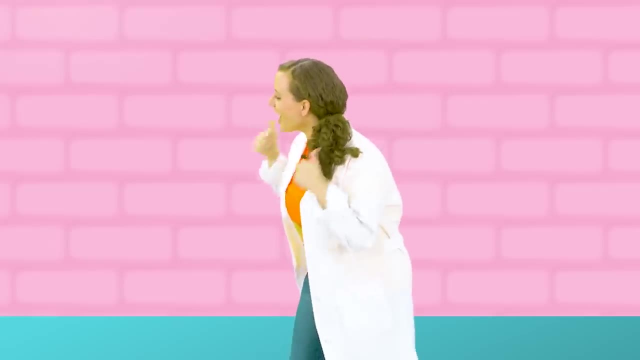 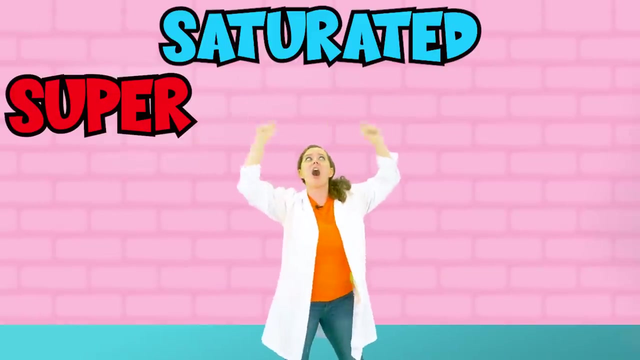 And then we're left with all this space that we can add a lot of sugar to. Hey, bring in the sugar. Look, Great job Pecks. Now that we have all this sugar, this is called a super saturated solution. As our solution cools, the sugar begins to crystallize. 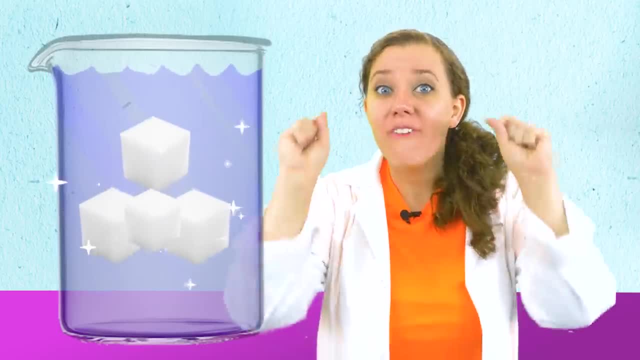 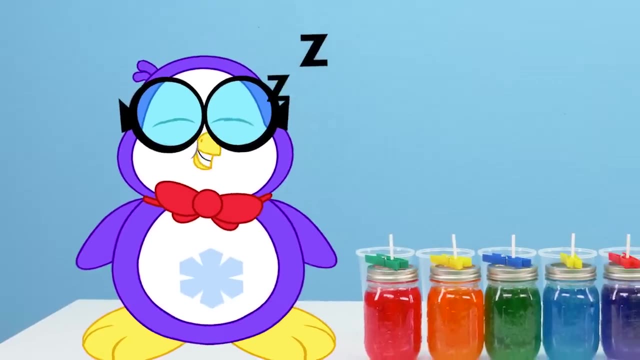 And these crystals form rock candy. Speaking of rock candy, I think ours is ready. Let's go. Let's go Candy. Oh sure, Peck, Peck, Whoa. Has it been 7,200 minutes? It has, which is why I'm here. 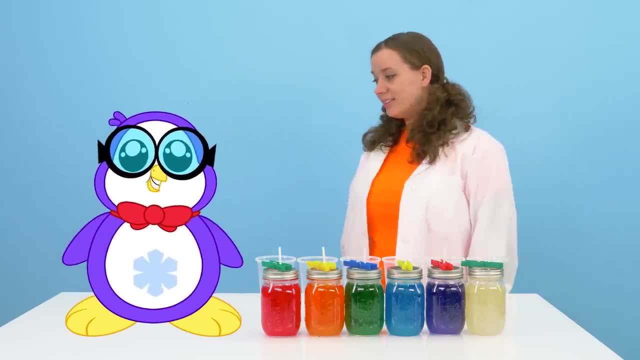 It's candy time. Candy, Candy, Candy, Yeah, But but how are we going to get the candy out? You're right, Peck. These are super saturated. They're going to melt, They're going to melt. 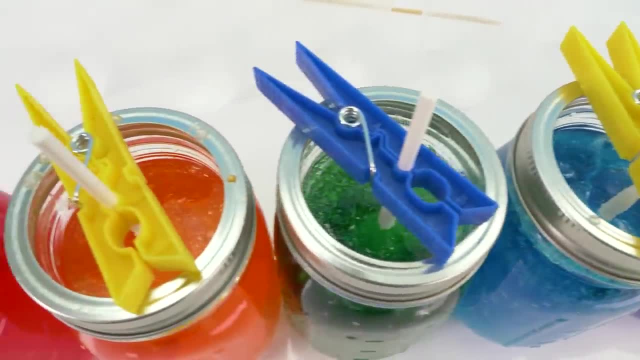 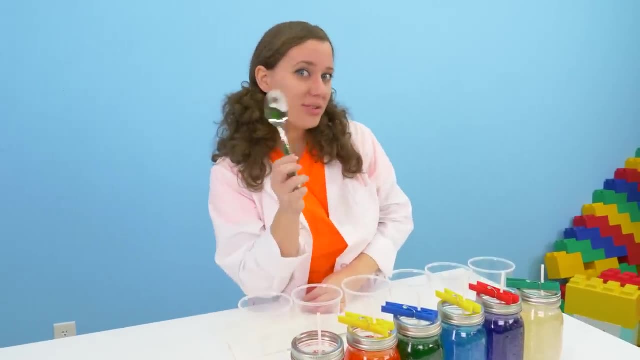 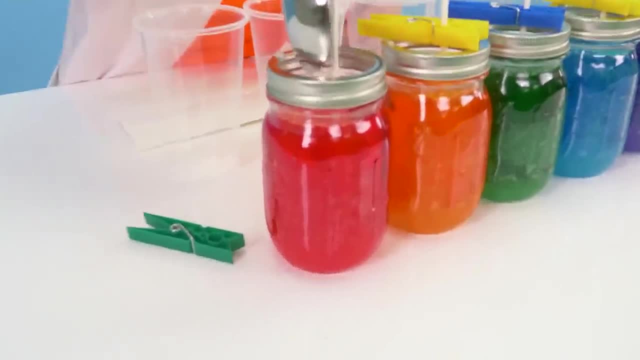 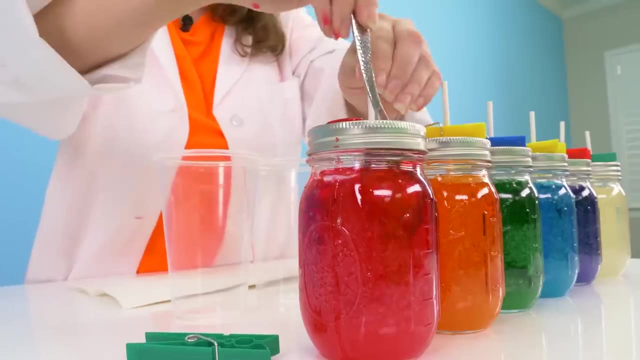 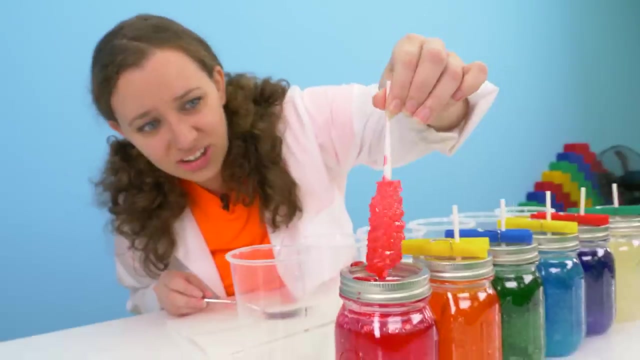 maybe chisel it out. So we need to break the top layer. Oh, my goodness, That is a lot of sugar crystals. Whoa, There we go. Oh man, it is all sugary and sticky and yummy. We definitely need this to dry. 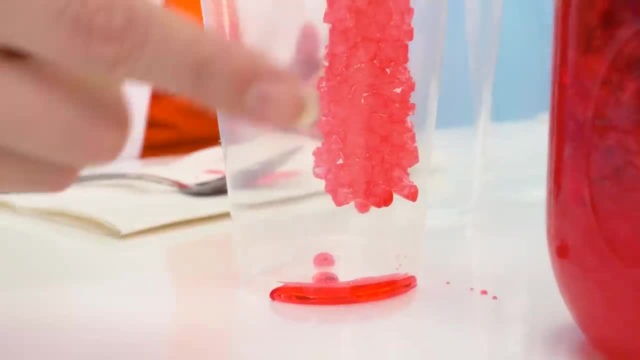 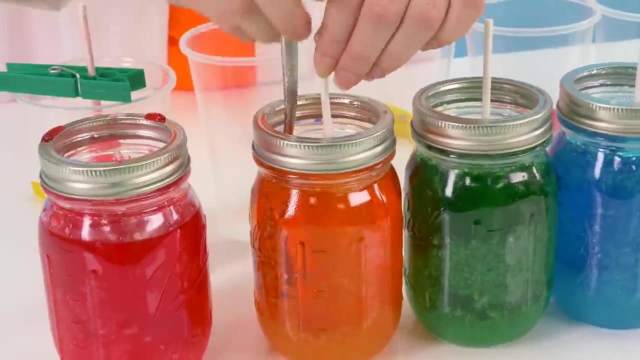 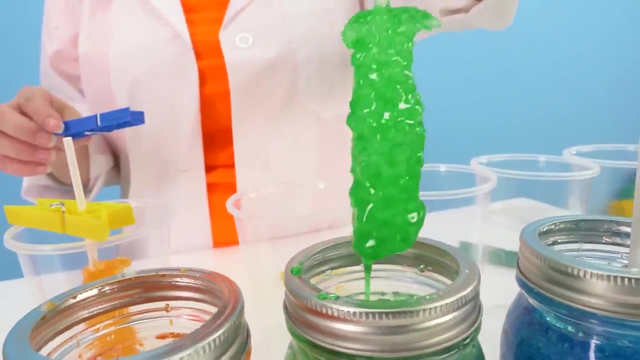 So we're going to use this cup to let our rock candy melt And remember to let your rock candy dry so it collects all this really sticky stuff And we don't make a mess everywhere. Oh wow, That looks so tasty and crunchy. 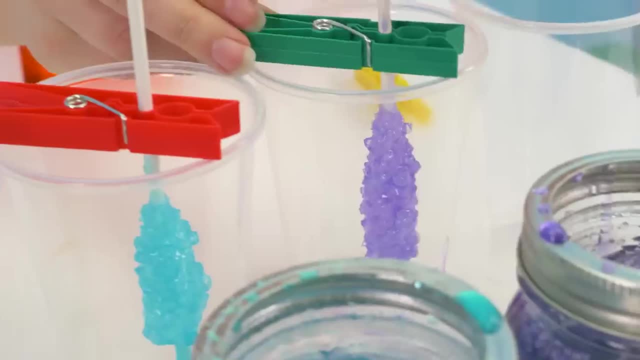 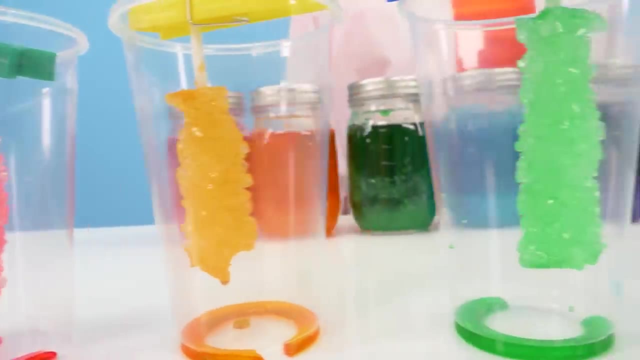 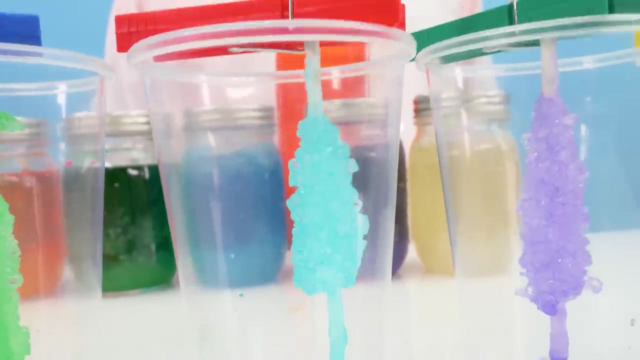 Phew, Got it. Oh gosh, I can't wait to try some. mmm, wait a second. that blue one looks broken. what happened? well, Peck, the stick got stuck in the jar when I went to pull it out, and that's because it was a little too close to the bottom. and all these? 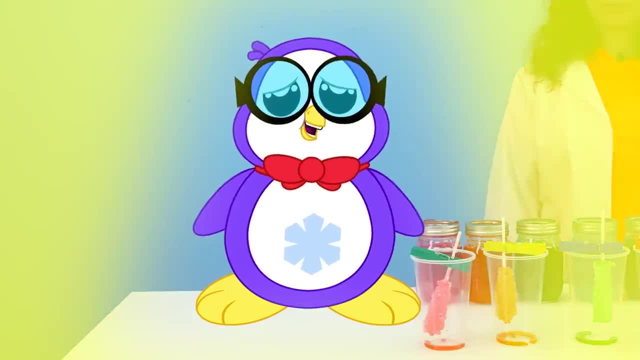 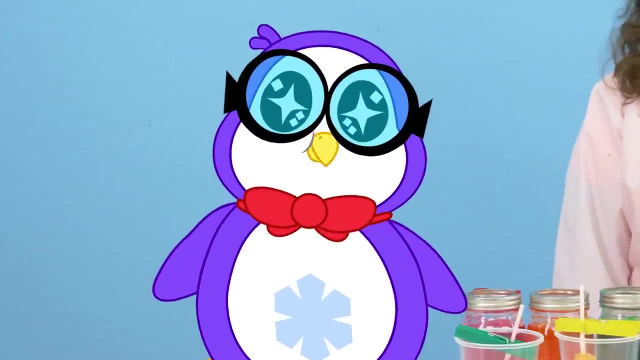 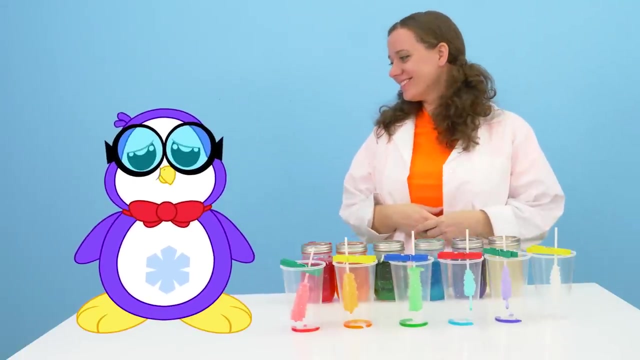 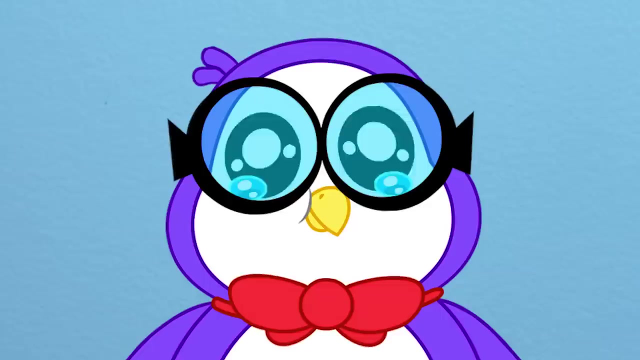 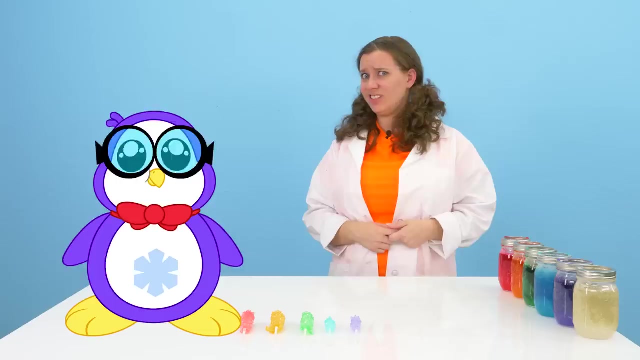 crystals grew around it. okay, if I try some of the candy now. I've been so patient and helpful. huh, we can definitely eat all of this rock candy really as soon as it dries, oh gosh, I can't take it anymore. Peck, the candy's ready. my patience finally paid off. yeah, sure good. 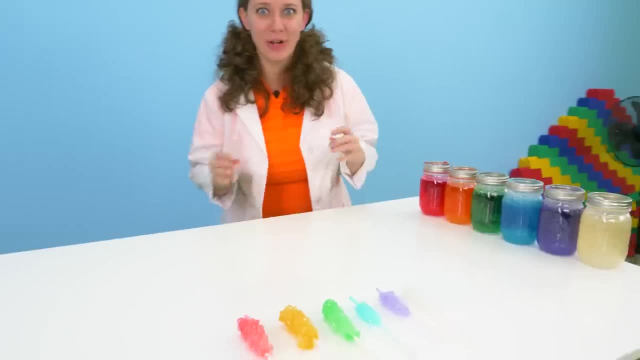 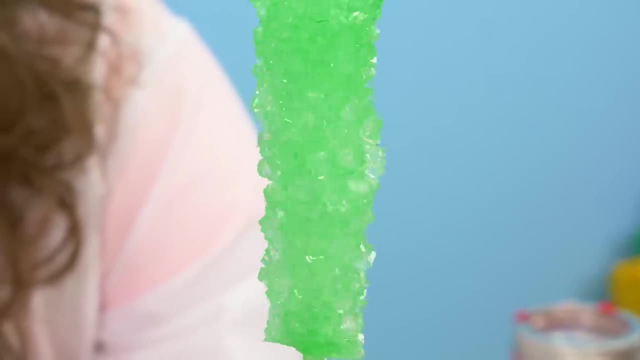 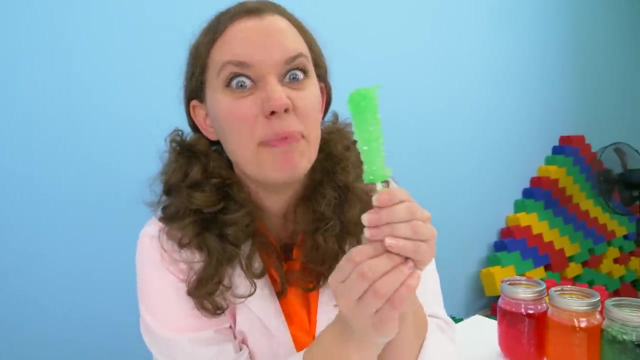 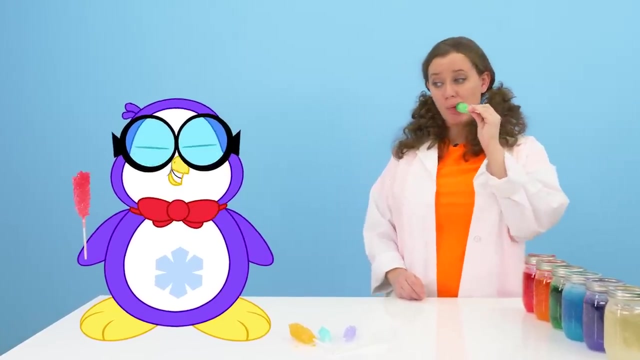 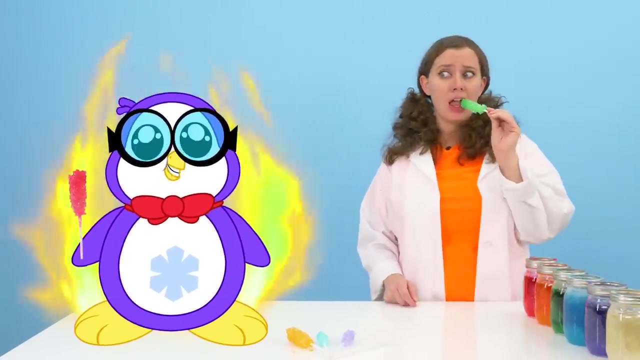 good job, Peck. now is the best part. we get to taste it. oh shiny. look all those crystals. they are so yummy and shiny. best part: mmm, that's really good. hmm, this is so good. it's filling me with energy, whoa. and the best part about this is it's so good. it's filling me with energy, whoa, and the best part about this is it's. 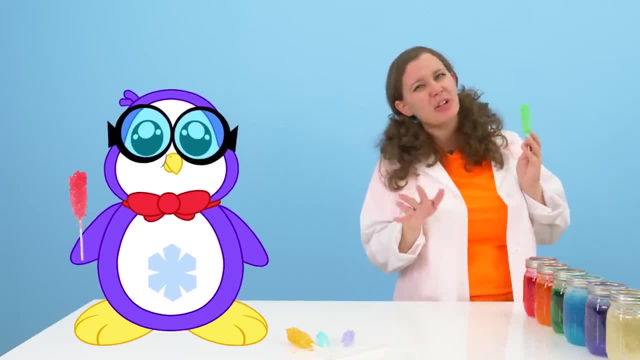 so good. it's filling me with energy, whoa. and the best part about this is it's so simple to make. you can make it at home too. it so simple to make. you can make it at home too. it so simple to make. you can make it at home too. it just takes a little bit, takes a. 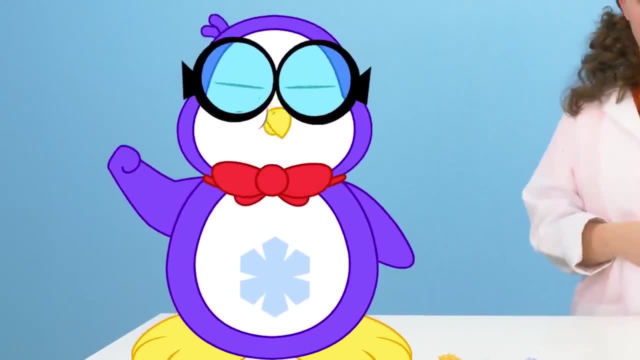 just takes a little bit, takes a just takes a little bit, takes a little while. yeah, I'm gonna eat the rest of little while. yeah, I'm gonna eat the rest of little while. yeah, I'm gonna eat the rest of huh. maybe it, maybe we'll we'll save. 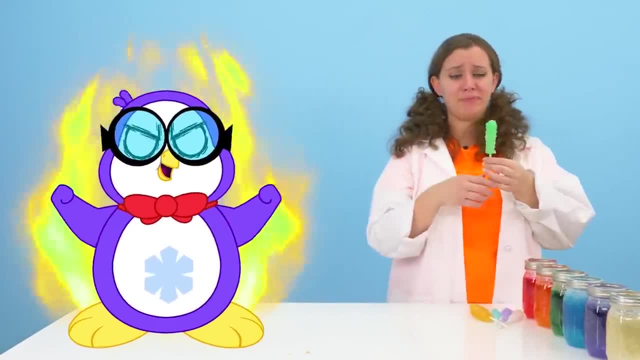 huh, maybe it, maybe we'll, we'll save. huh, maybe it, maybe we'll. we'll save those for later, Peck. okay, thank you for those for later, Peck. okay, thank you for those for later, Peck. okay, thank you for showing me how to make these rock. 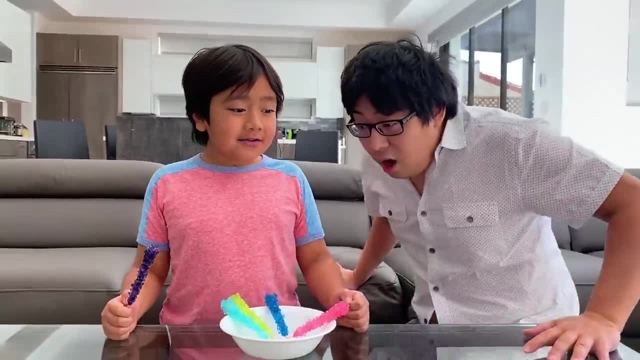 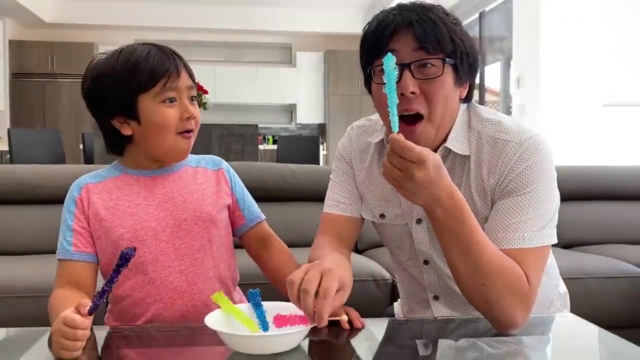 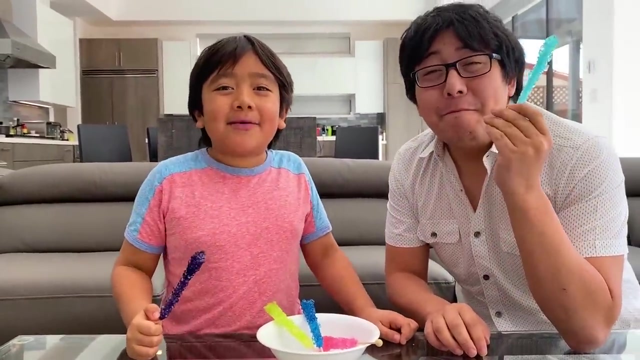 showing me how to make these rock. showing me how to make these rock candies. it's so cool. you want to try rock candies? it's so cool. you want to try rock candies? yeah, and it is great. oh so candies, yeah, and it is great. oh so candies, yeah, and it is great. oh so sweet. thank you for watching our how to make.